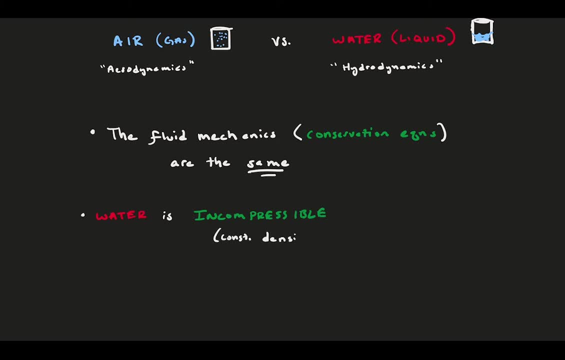 constant everywhere in the field and that significantly simplifies the math. air, however, is often compressible, especially in high-speed flight, and this can make the math more difficult and causes us to need more equations, like the conservation of energy in the equation of state to find all the 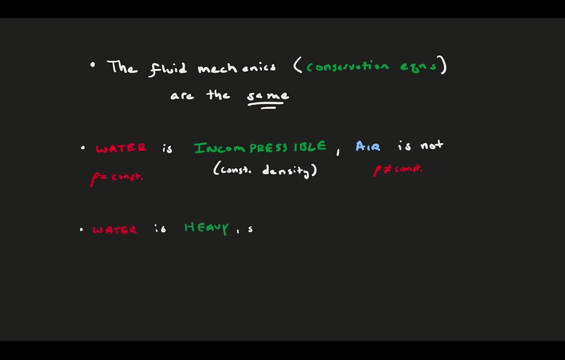 variables. second, water is quite heavy compared to air. this means that in order to be held up in the water, it is easier to use the buoyancy force, but in order to stay up in air, we need to generate a vertical force, which is known as lift. think of it this way: a neutrally buoyant fish really needs to only worry. 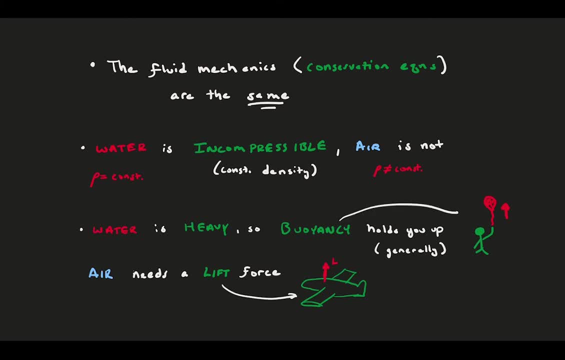 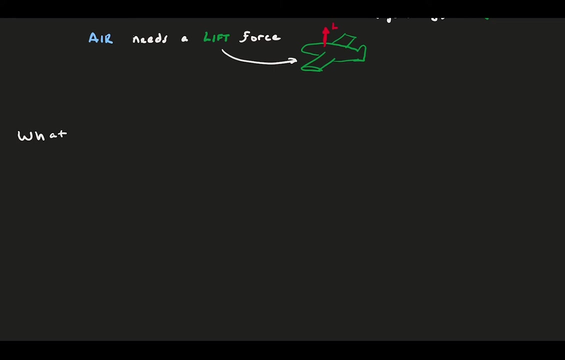 about using its fins to move forward. a bird, however, needs to worry about generating lift to stay up while simultaneously generating force to move forward. so these unique aspects of moving through air and the usefulness of air transportation are the reason we have specific courses dedicated to it, and once you've learned aerodynamics, 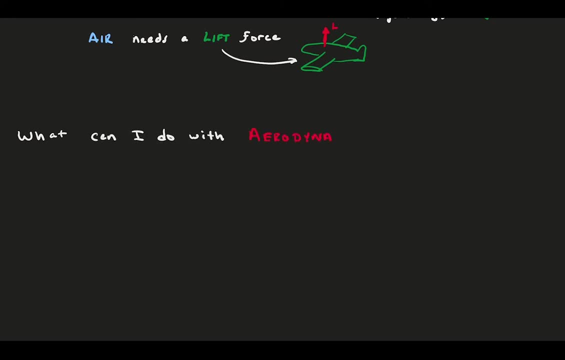 there's a ton you can do with it. obviously, aerodynamics experts are needed in the design of aircraft. commercial aircraft, uncrewed area vehicles, fighter jets- all foundationally operate on aerodynamic principles. automobiles heavily rely upon lowering air resistance to decrease fuel consumption or improve race time. 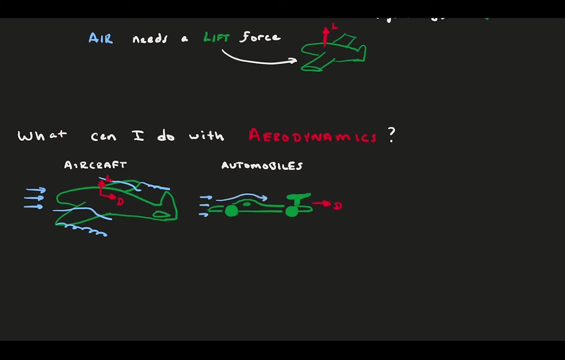 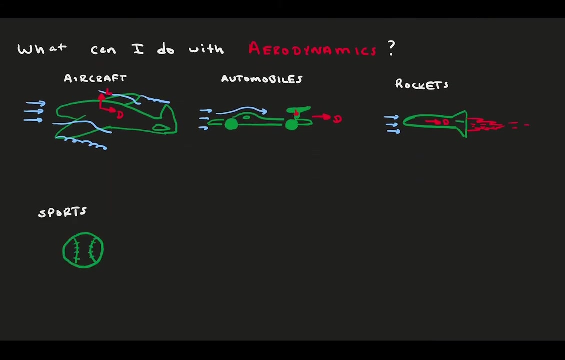 rockets and ballistics often reach hypersonic speeds and rely on aerodynamics to know where they are going and to get there accurately. aerodynamics- aerodynamic forces, show up in countless sports, including the cycling to lower air drag, or golf and baseball to manipulate the flight dynamics of the 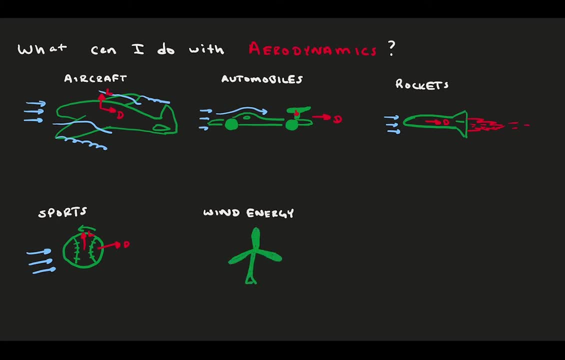 ball. some people use aerodynamics to save the planet by designing technologies to harvest wind energy. and, lastly, in order to get to the vacuum of space, you have to travel through the atmosphere, which can be tough with such high altitudes and low air density. aerodynamics. 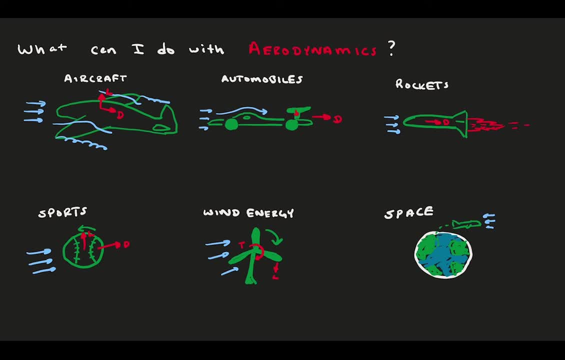 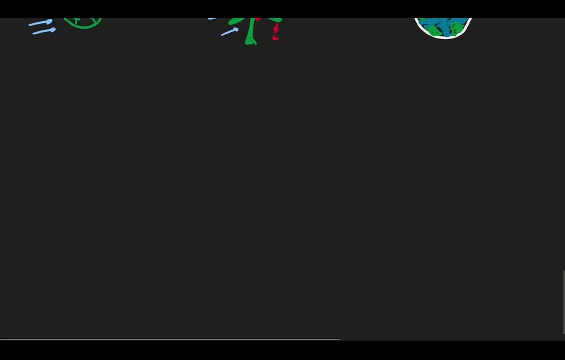 so knowing and specializing in aerodynamics opens up a wide variety of interesting career opportunities. now that I've hopefully convinced you we should want to study aerodynamics, how do we do it specifically? let's consider how studying aerodynamics is different than how we would approach fluid mechanics. let's consider an object in an airflow in this, 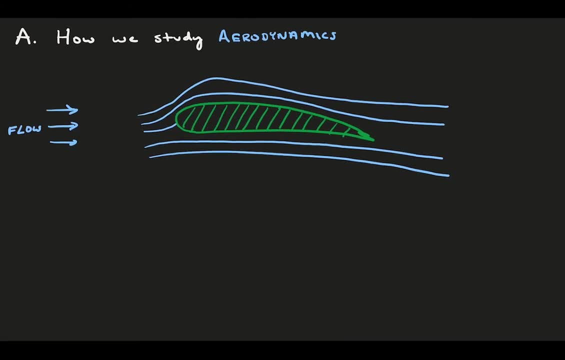 case in airfoil. first, aerodynamicists are generally concerned with the global body forces that the flow causes. consider the way a fluid mechanician would study this type of flow. they would be very concerned with defining the exact flow field as it develops over the object. in general, they would seek a mathematical definition of 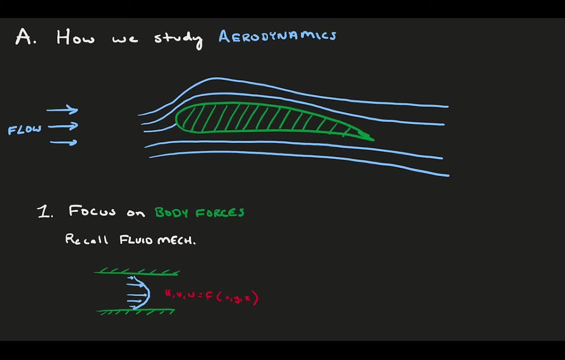 the entire flow in aerodynamicists would approach things a bit differently. their primary concerns are the body forces produced, things like the overall lift and drag, the moments produced, specifically if body forces are generated from away from the center of gravity, and the pressure distributions that produce these body forces, and 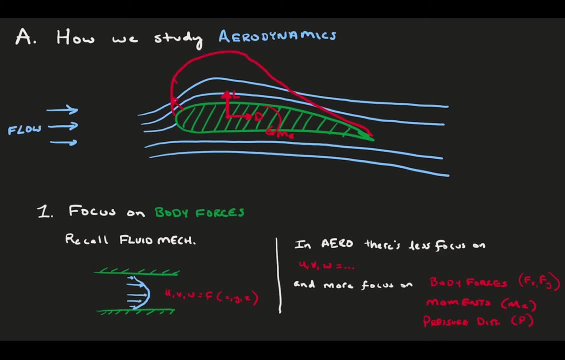 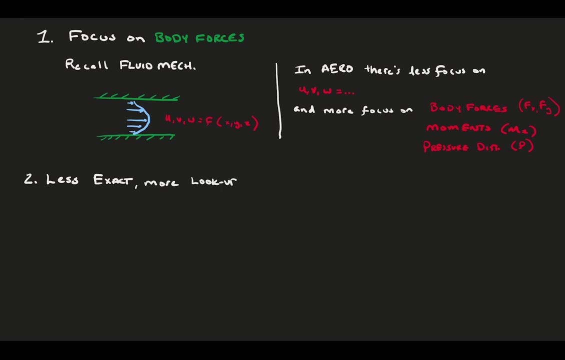 moments. in order to get to these body forces, you do need to know something about the flow itself, but you can do more estimating and modeling to predict these forces. as a result, aerodynamics is much less exact than how we approach fluid mechanics. in fluid mechanics, the conservation equations are solved exactly, or? 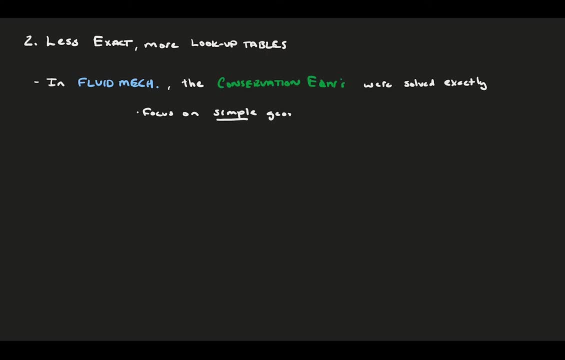 approximately given a very simple geometry like a channel, a pipe or a flat-plate boundary layer in aerodynamics we generally can't arrive at the exact flow in aerodynamics. at exact solutions. The geometries are much more complex. There are a wide variety of airfoils of 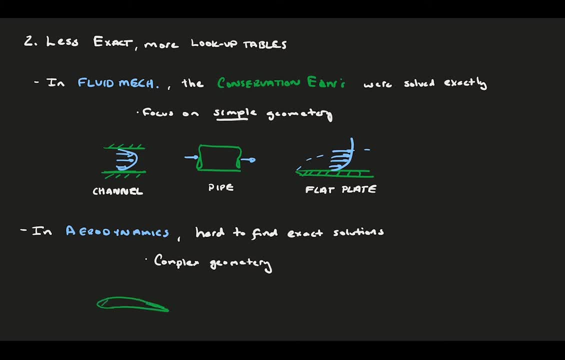 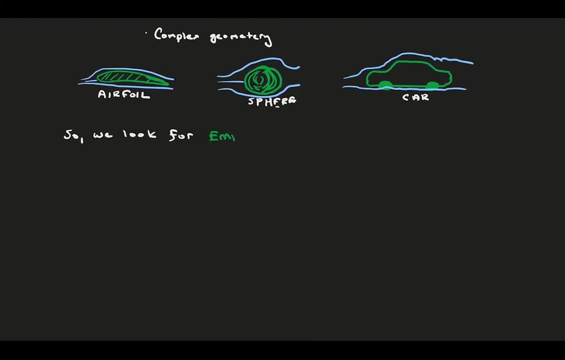 arbitrary shape spheres with three-dimensional separation and a wide array of ground vehicles that can change the flow behavior. So we do a lot more looking things up in documented tables that have empirical values. For example, let's say we have a plane flying at some velocity and 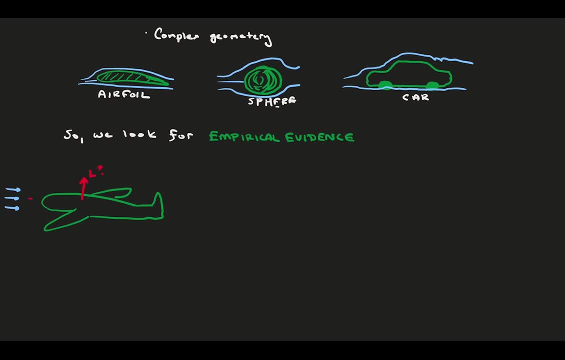 angle of attack that we know. How could we know what lift it's generating and making sure it can stay in flight? In this case, there's way too much going on to solve the flow field everywhere. So what we do is we mark down the meaningful parameters like flow speed, angle of attack. 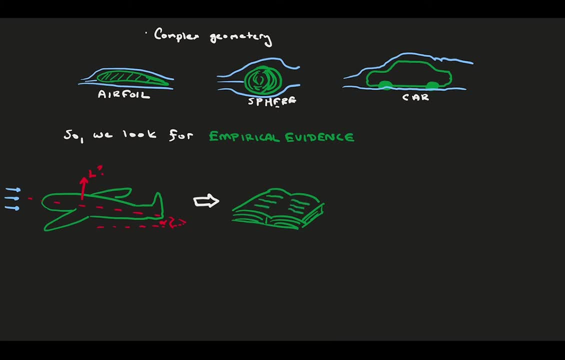 and what type of airfoils we're dealing with. Then I take out a reference that has pages of tables where people have documented what forces they found when they put an object like this in the flow. You then find the table with the parameters that matter for you, like the airfoil type and flow. 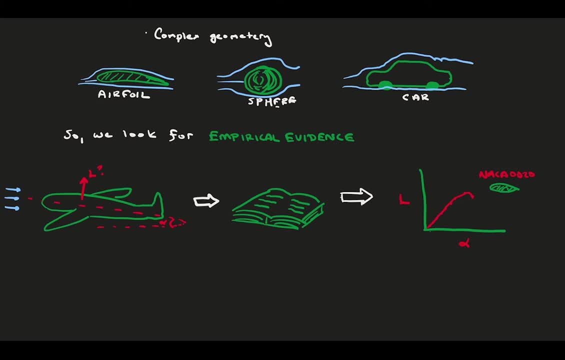 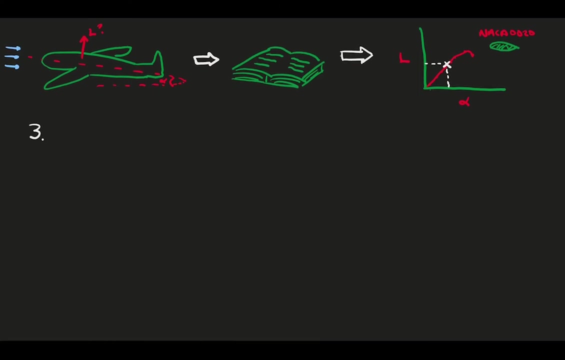 speed and you look up the approximate lift you would expect to see at that angle of attack. With some work, you can then apply this to the entire plane and ensure that your lift is sufficient to maintain flight. While we care about the body forces generated by the flow, we're also interested. 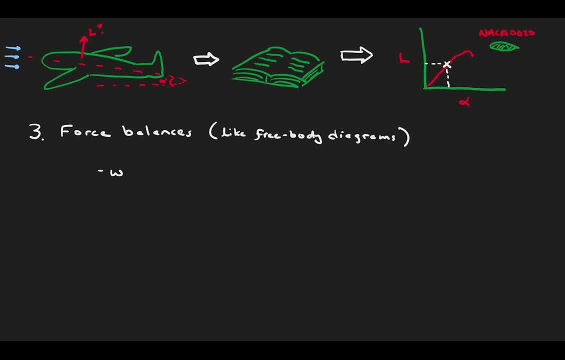 in the entire force balance of a vehicle, Much like a free-body diagram. When an object, like a plane, moves through the air, it experiences a number of forces in various spots. Generally, our goal is to move steadily, meaning no acceleration or deceleration in any direction. In order to maintain steady flight, we need to counter. 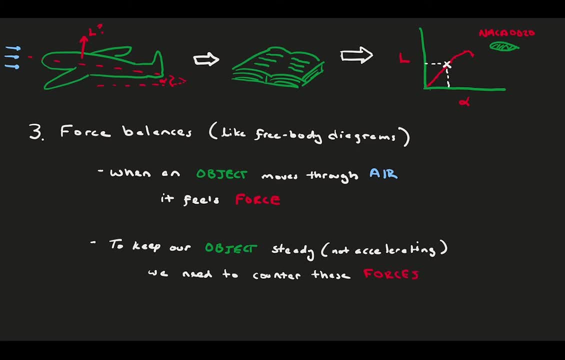 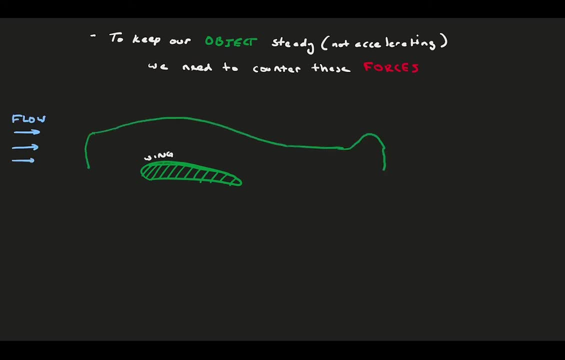 the forces from the air. Consider a wing attached to a plane. As the plane moves through the air, it experiences lift which is perpendicular to the flow velocity. In order not to fall out of the sky, the lift must equal the vehicle weight. Similarly, 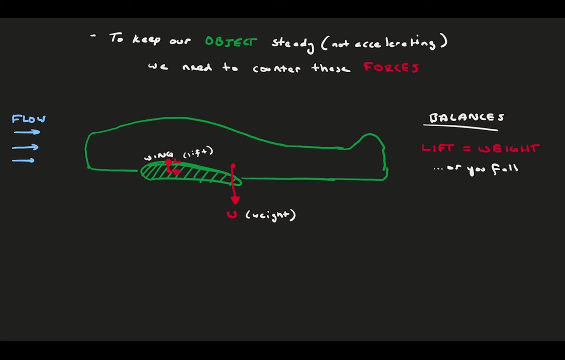 the air force along the flow direction is the drag force. To counter the drag we need thrust. Often the thrust is produced by a turbine, a propeller or a burning propellant. If the drag and thrust are not equal, we either speed up or the thrust is produced by the 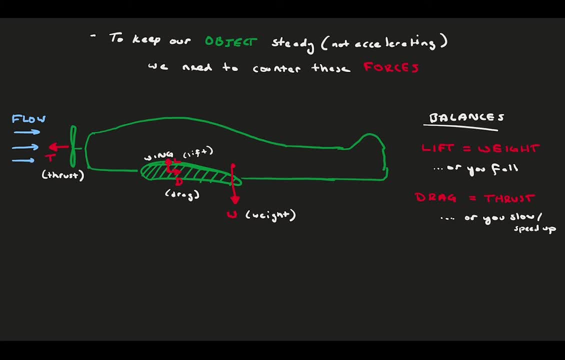 air. In order to maintain steady flight, we either speed up or we slow down in the flow direction. Additionally, the central location where the body forces act on the foil can change depending on the flow conditions. This causes issues, because then the lifting force produces a. 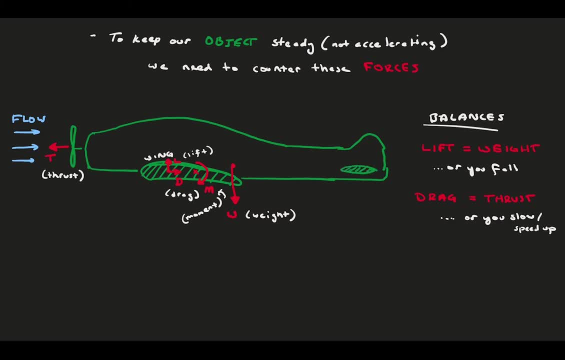 moment about the plane's center of gravity inducing rotation. If we want to maintain steady flight and not do backflips, we need to create a force that counters this moment, which can often be done at the tail of the aircraft. The tail has a different airfoil with different lift force. 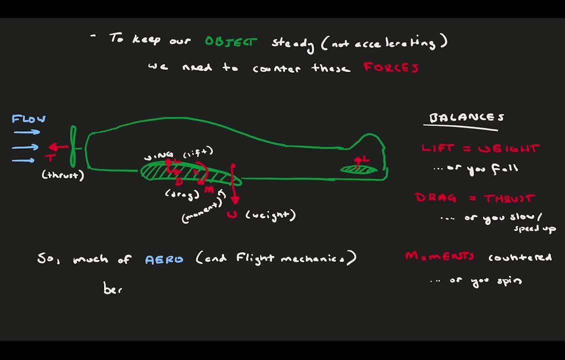 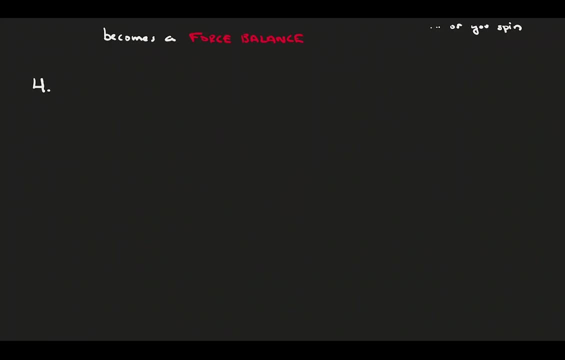 So you can see how aerodynamicists need to know a bit about the fluid mechanics, but they also need to keep the forces on the entire vehicle in the back of their mind as they do their analysis. And finally, in aerodynamics we end up needing to solve for more flow variables, The velocity, 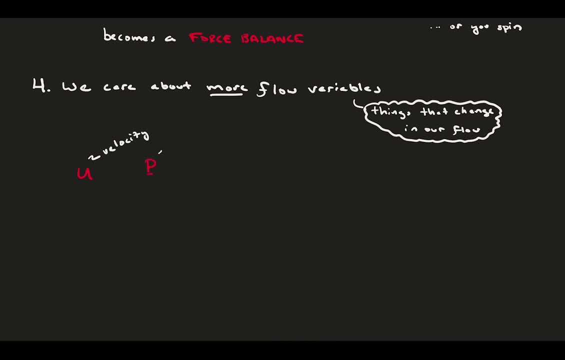 field and the pressure field are the main players in introductory fluid mechanics courses. The velocity field and the pressure field are the main players in introductory fluid mechanics courses. In order to solve for the velocity and pressure, the two unknowns, you need two equations which: 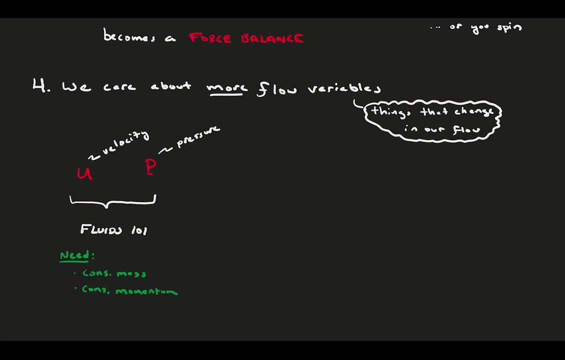 end up being conservation of mass and momentum For the majority of fluid mechanics until you explore compressible flow. that's about it. However, in aerodynamics we often need a few more flow variables, especially in high speed or high altitude flight. 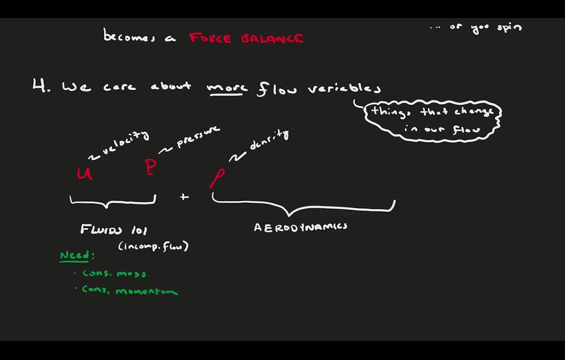 First, the density in air can vary a lot more easily than it can with other fluids, So that means we have an additional flow variable. In addition, there is an additional variable to solve for, as well as another equation, And this equation is generally the conservation of energy. 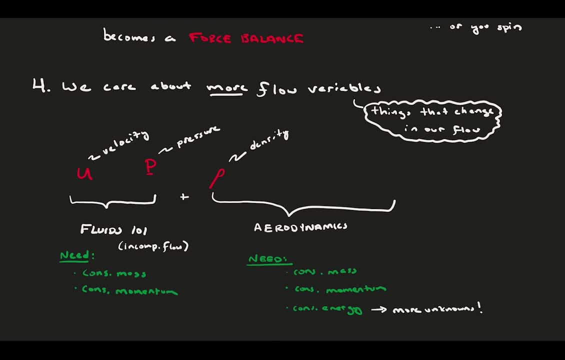 Unfortunately, when we introduce this new equation, we get more unknown variables. Specifically, we add the unknown of internal energy as well as temperature and temperature. Two more unknowns means needing two more equations For the types of unknown variables. inIEpot molecules. 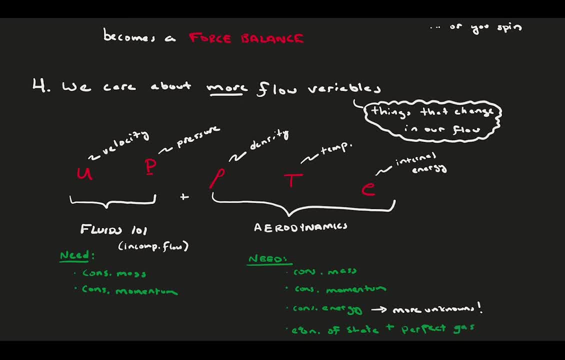 we can work them out in a lot easier way than what we know as the boson equation, Which leads us to the equation of state in the perfect gas equation. In the end, we have five unknowns in five equations. So in edequation, we have twoочно of state- �ية 2017, and in kical of state, we have an white p' of z. 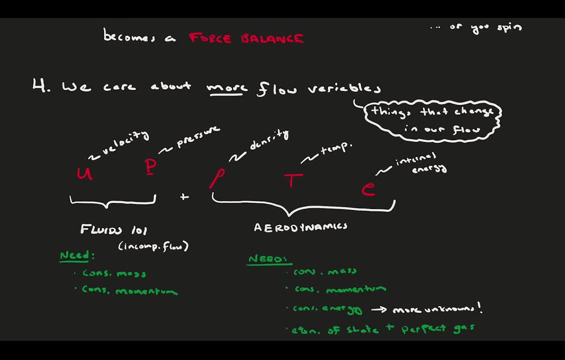 in five equations and solving for all of the unknowns becomes a bit more difficult. Outside of the equations, it's important to note that, from an engineering perspective, knowing the temperature in a lot of aerodynamic vehicles is absolutely critical. Reentry vehicles get super hot, so hot in fact.